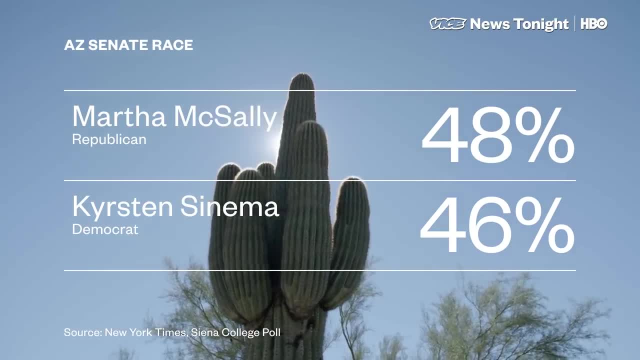 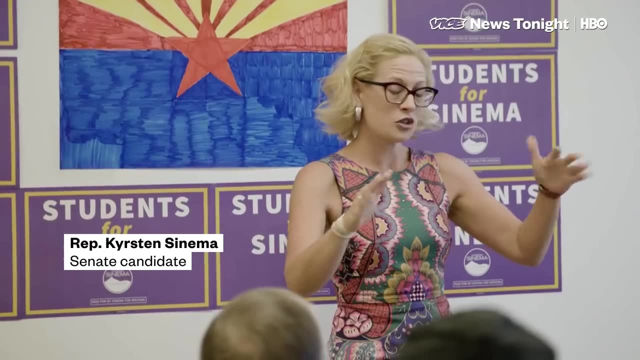 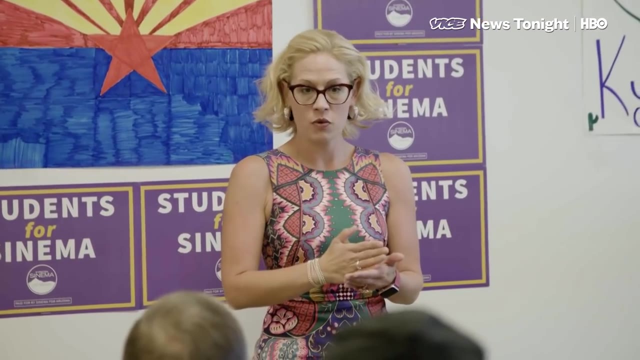 This year there's a competitive Senate race And Democrats are already running their Get Out the Vote or GOTV program. Their focus is the early vote. What we've got to do between now and the next 18 months is work, work, work, run across that finish line. run faster than we've ever, run, harder than we've ever run. 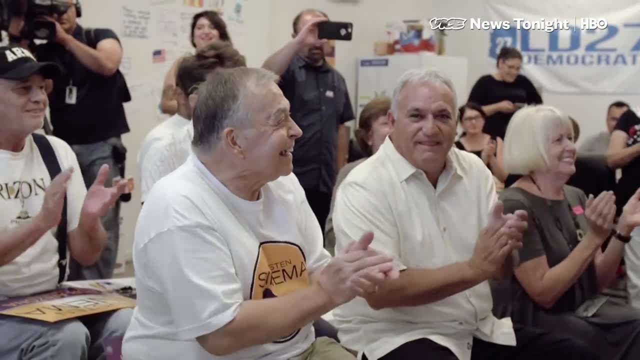 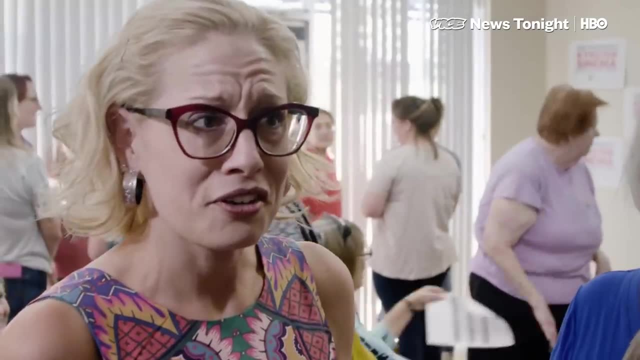 That's how we're going to win this race. Thanks you guys. Thank you. How do you get people to turn out and vote early and why do you want them to? You're not from Arizona, I'm not. Yeah, okay. So right now in Arizona, early voting has been going on for over a week. Eighty percent of Arizonans will vote before the actual Election Day. In Arizona, the ballot is very long, Yeah, So you get plenty of time to consider and vote. 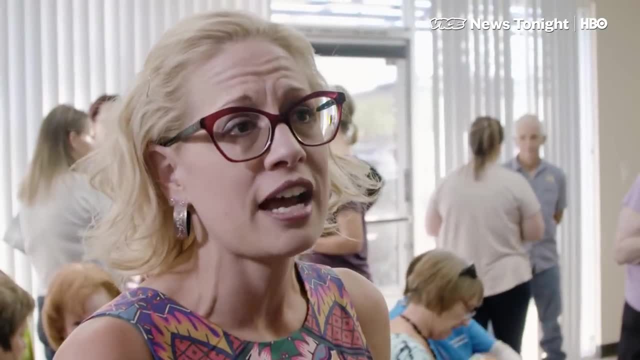 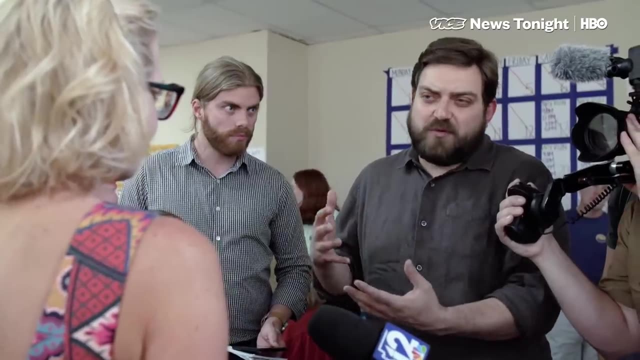 That's how most Arizonans vote. It is hassle-free and allows them to have the time to make their decisions in the comfort of their own home. But, like for your campaign, doing a GOTV here, at the end it's more helpful to have. 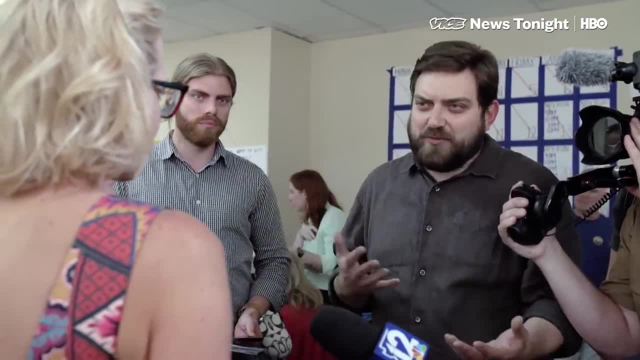 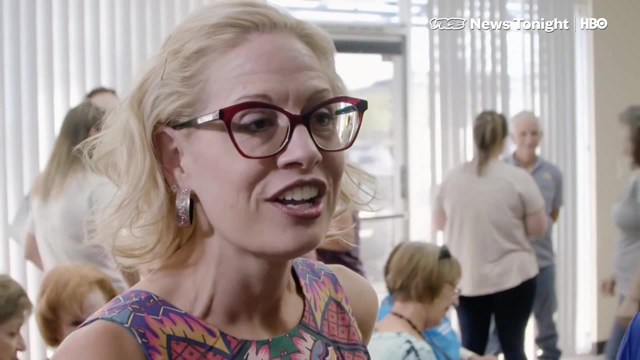 people vote on the front end than on the back end of that period. Does it matter when people vote? Well, we want everyone voting as early as possible because once your vote has been sent to the county elections department, you know your vote is secure. 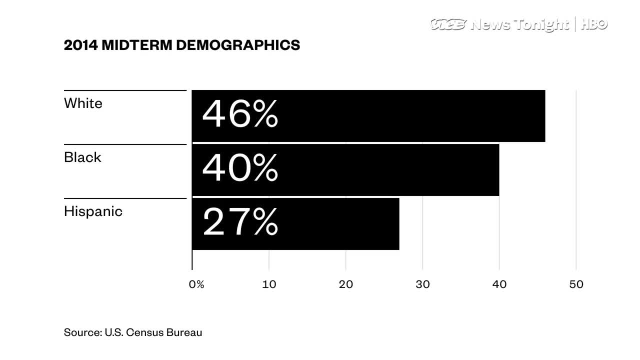 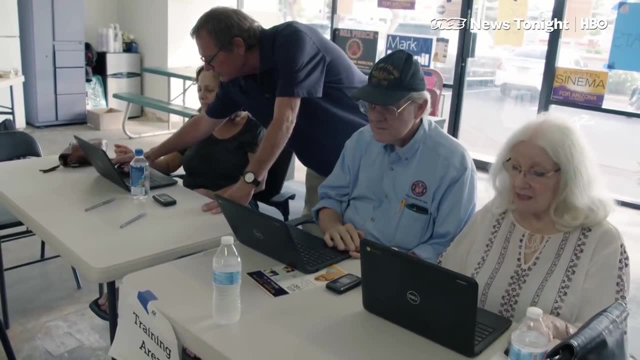 Midterm turnout is generally more of a Republican thing. Older, whiter, richer voters go to the polls without much prodding, making it much easier for the GOP to put numbers on the board. Democrats have a tougher time. They often rely on voters who may have never cast a ballot in a midterm. 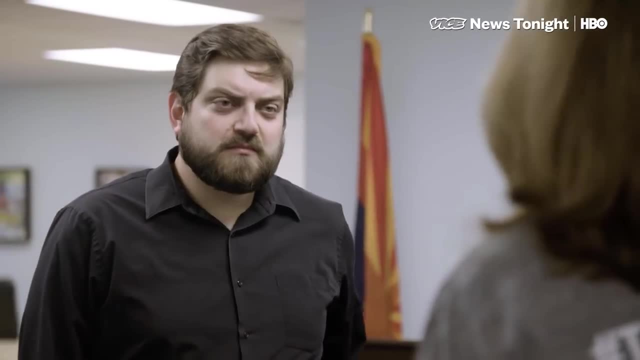 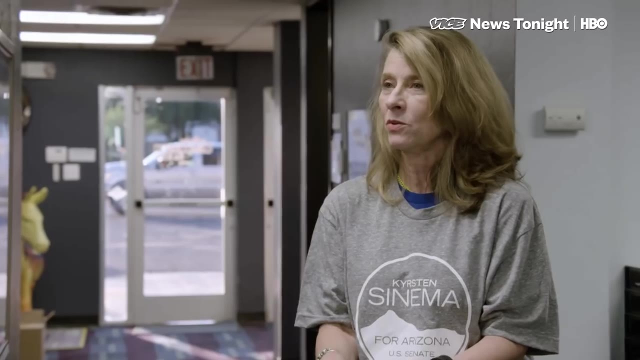 Early voting is very helpful for brand-new voters. Let's say, this voter is a student or a working mom or has a new job or has just moved to Arizona. These are all ways that voting is just not going to be on their radar. Yeah. 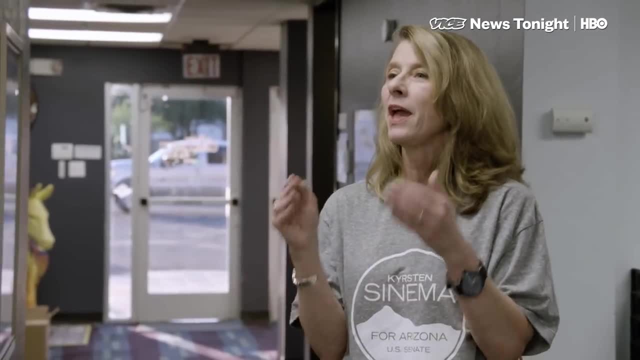 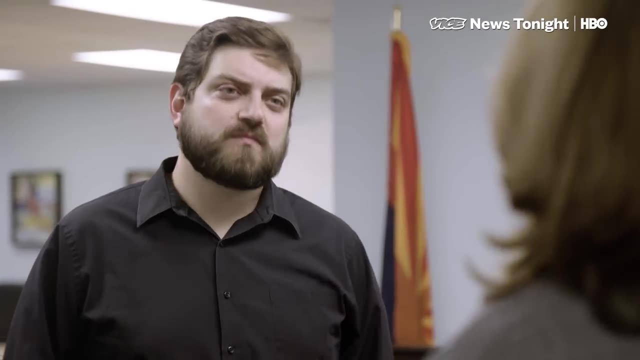 We get them to pay attention when it comes in their mailbox and they know they have this opportunity and a duty to vote, There's a less likelihood of voter suppression for folks who vote early. They're already on the voter rolls. They already have gotten their ballot. 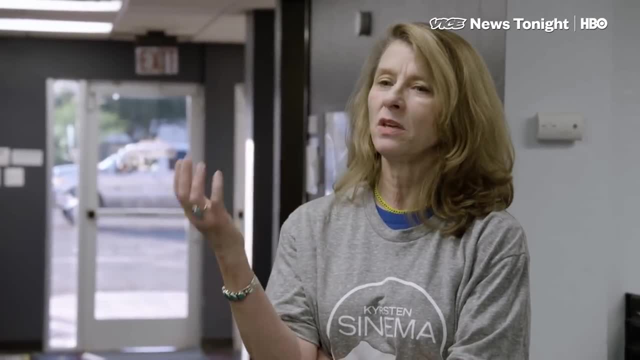 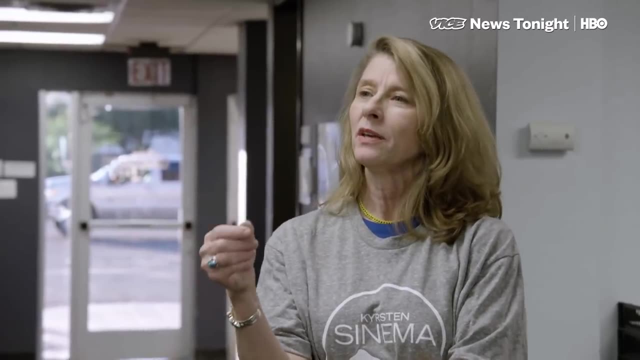 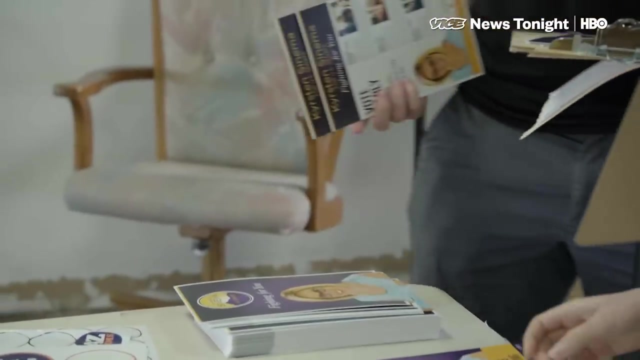 When you go into the polling locations, there can be issues about addresses and changes of address and things that cause folks to be put on a provisional ballot. This way, everyone has a greater chance of getting a vote. Everyone has a great shot at getting their vote counted. 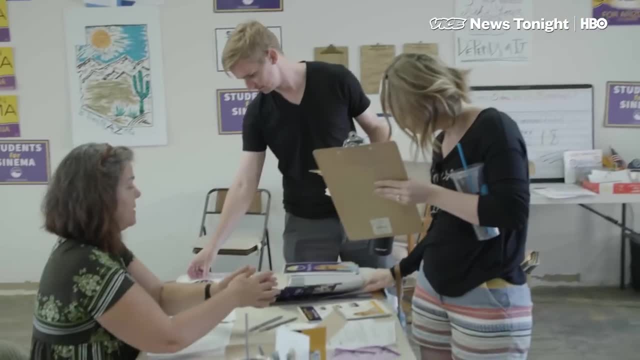 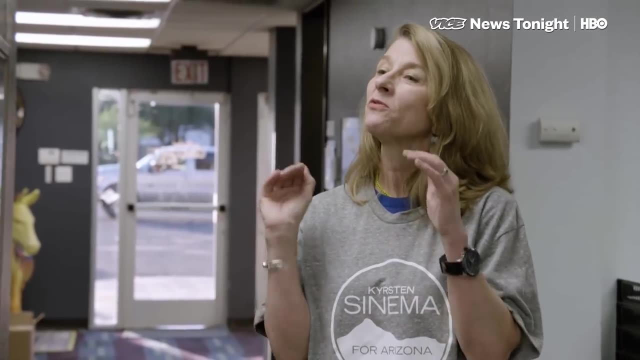 Democrats turn on operations get a benefit too, Because early voters are easier to track And bank When we see the data coming in. then we can be more efficient in how we get the vote out. Once we know who's voted, we're going to leave those guys alone. 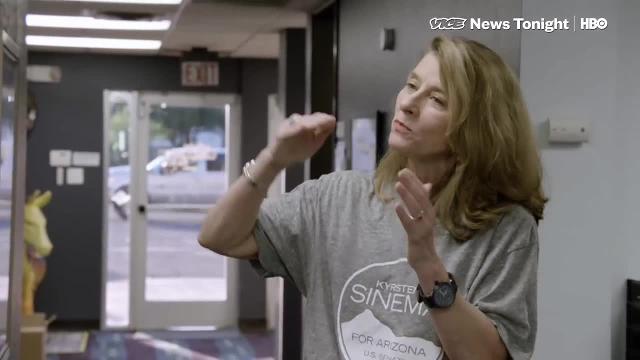 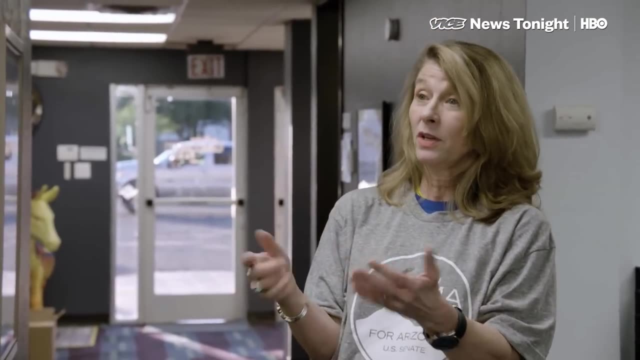 And then we're going to go and look at those lower-efficacy voters and start calling them, going to their doors knocking and asking them if they've got their votes. Are they going to get their early ballot And are they going to vote? 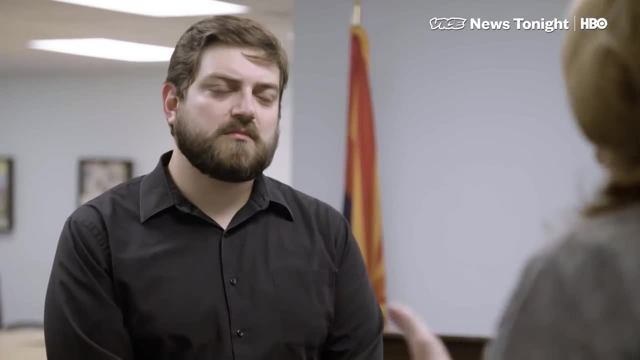 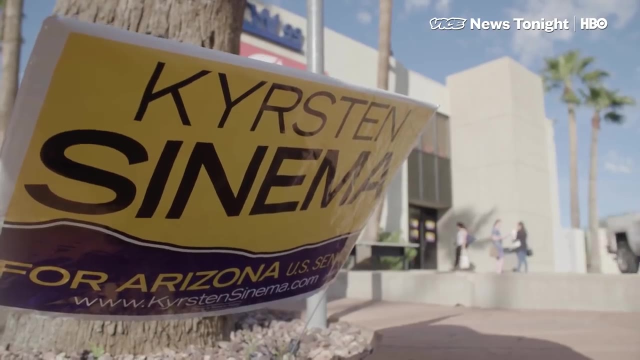 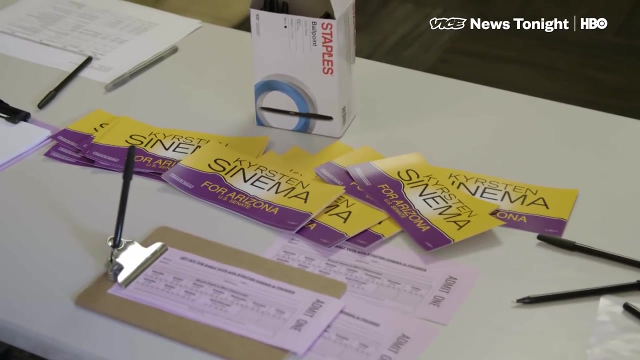 So the data tells us the trending and, in the midterm cycle, who is voting and how likely a voter is to vote is really important. Weeks ago, the party pushed people they expect to vote Democrat to request mail-in ballots. Now they're tracking who sent those ballots in. 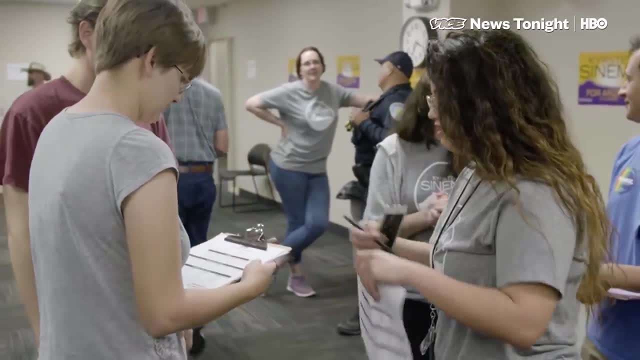 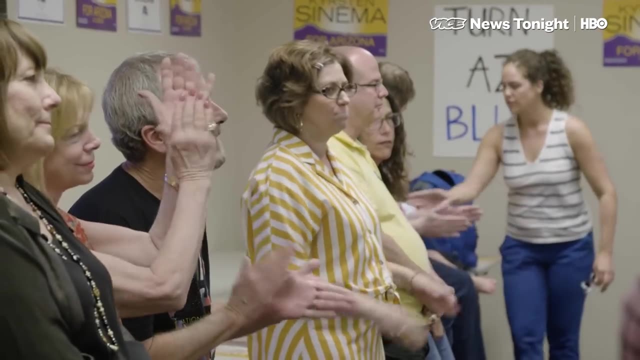 It's precious knowledge because it means that on Election Day, Democrats won't be wasting time on voters who already voted. Is the strategy working? Depends on who you ask. In Florida, state Democrats are touting the early returns from mail-in votes. 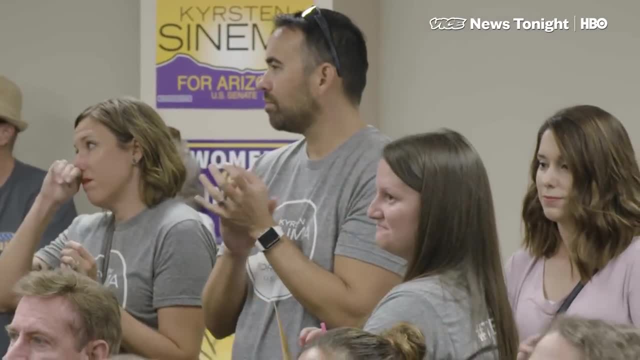 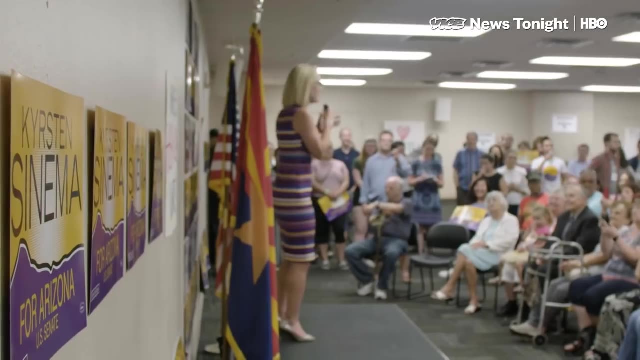 They show first-time Democratic early voters are actually showing up Here in Arizona. the party's talking about huge registration gains and the number of ballots that have been requested. What they're not saying yet is that they're winning the ballots that have been sent in. 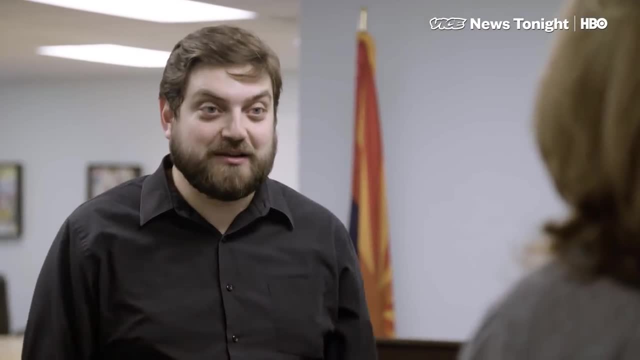 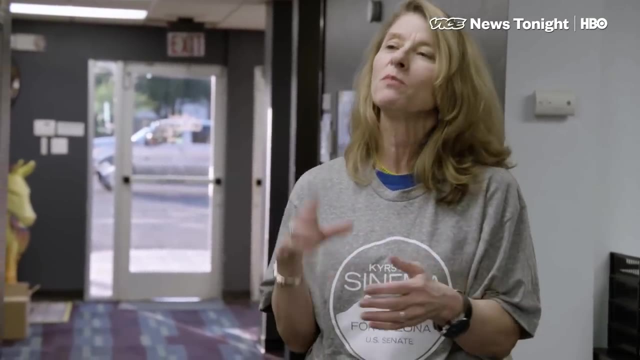 If Democrats win in Arizona, will it be going to be because of early voting? sounds like It will be a big piece of it, Because people who know who they want to vote for are going to vote early and people who need to take a little more time to do the research are also going to vote early. 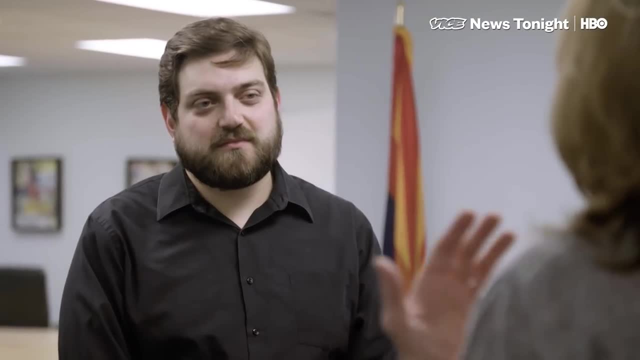 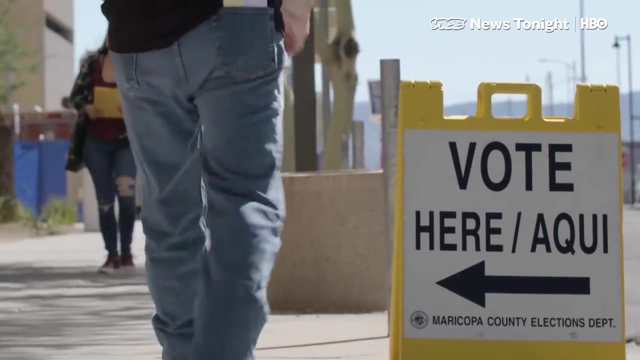 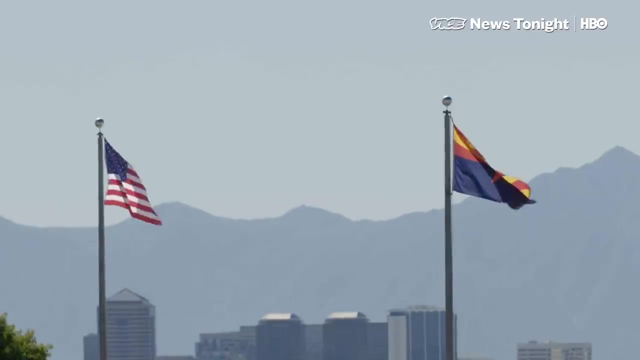 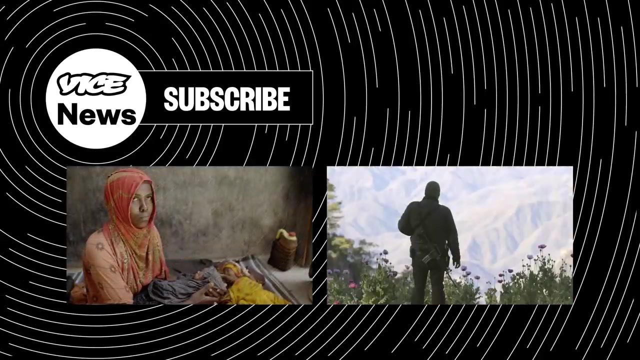 because they've got the opportunity to do so And we believe that when our Arizona voters- Republican, Democrat, Independent- go to look at who they should vote for, they're going to pick Democrats And they're going to do it for where they're common interests. 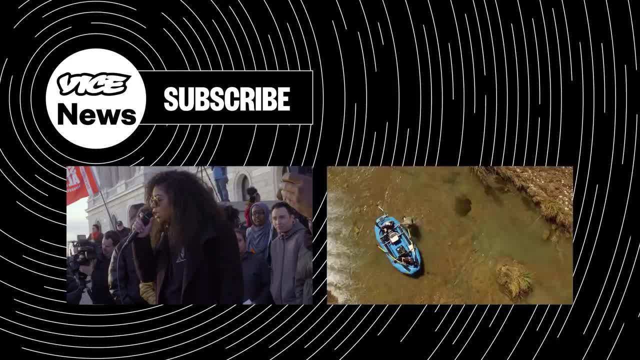 So basically, it doesn't even show who's in a ministerial seat right now, And we're obviously going to have to move these groups until they'reưởng bigger than just Karen Hays. All right, Thanks everybody. Thank you for being here. You've been fantastic. I enjoyed it And look for the next few time time once again.